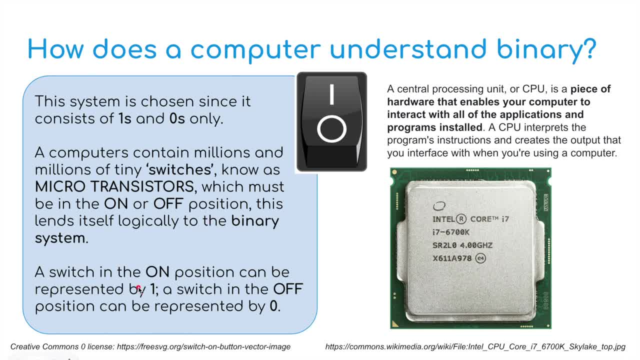 This lends itself logically: The binary system. a switch in the on position can be represented as a one, like so a switch in the off position can be represented as a zero, like we see here. This picture here. this is an example of a CPU, the brains of the computer. 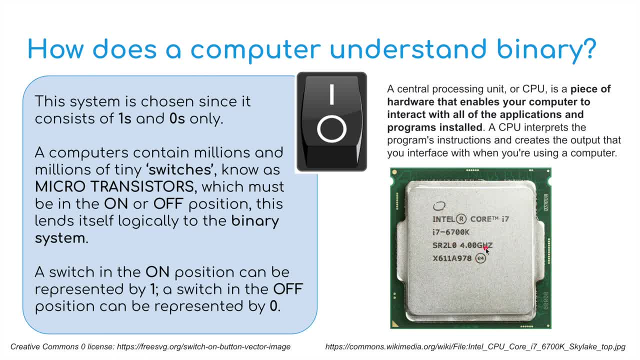 In this CPU, the central processing unit. it's a piece of hardware that enables your computer to interact with all the applications and all the programs that are installed on your computer. A CPU interprets the program instructions And creates the output that you interface with when you're using your computer. 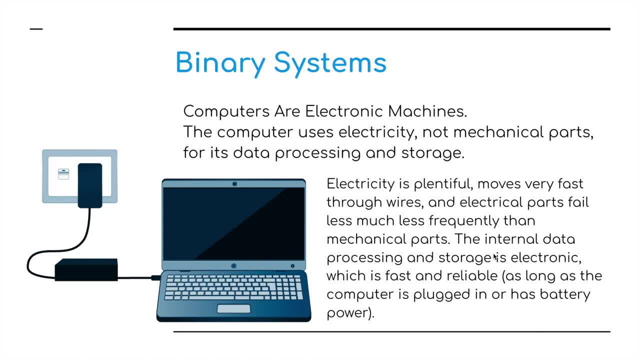 So binary systems. computers are electronic machines. We can see that it's plugged in here. Normally a laptop has a battery or it's connected to the mains. The computer uses electricity, not mechanical parts, for its data processing and storage. Electricity is plentiful, moves very fast through wires, and electrical parts fail less, much less frequently than mechanical parts. 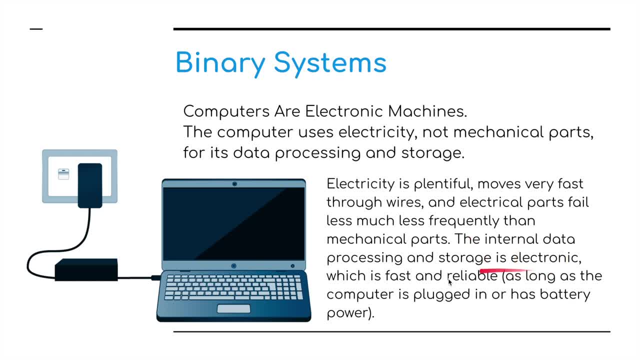 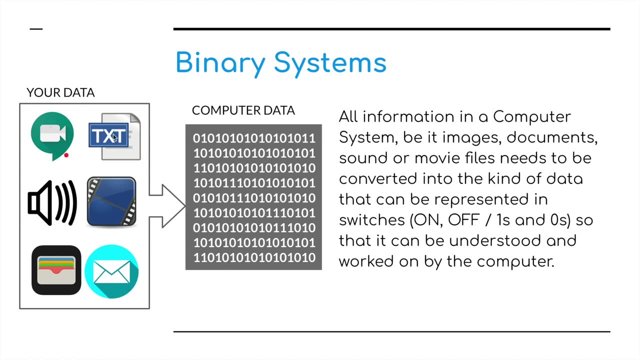 The internal data processing unit is a computer- The processing and storage is electronic, which is fast and reliable as long as the computer is plugged into the power or has a battery power pack attached to it. Here we can see your data, whether that's messages, whether it's text, sound, movies, whether it's your Apple wallet, whether it's emails. 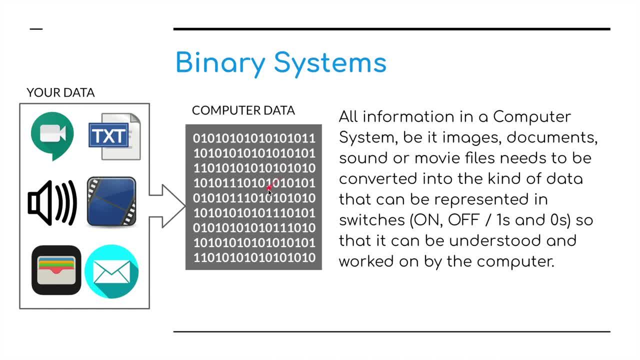 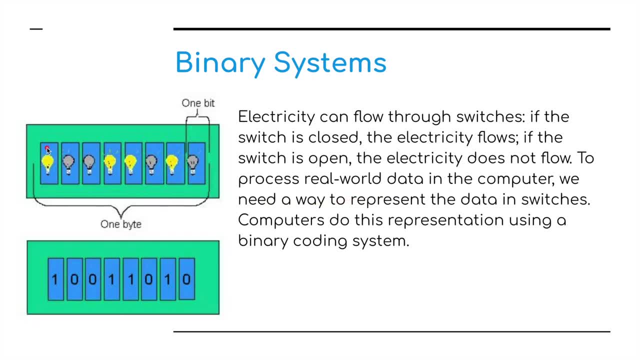 All of these, in order to work on a computer, get converted into binary values, into binary data, So binary data can be used to convert data into a computer. We have here what they call a byte of information. Each of these blue rectangles we can call a bit. 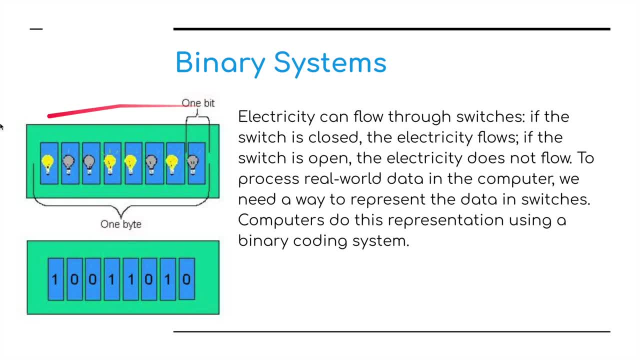 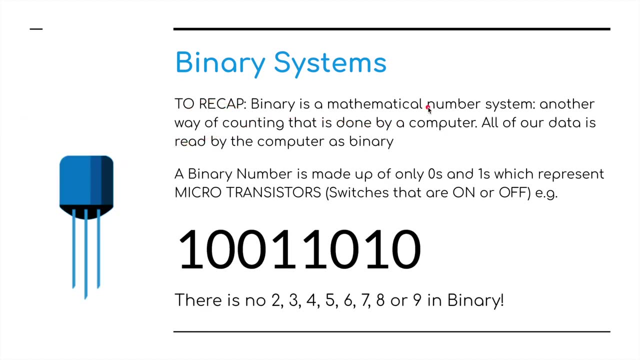 There are eight bits, which equals a byte. Eight bits in one byte. B-Y-T-E. OK, if the value is zero, it is off. If the value is one, it is on. To recap, binary is a mathematical number system. 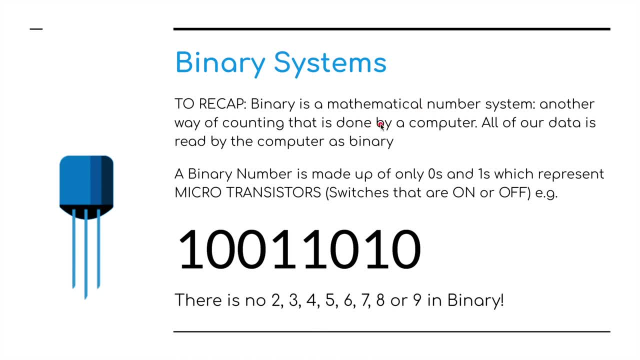 Another way of counting that is done By a computer. all of our data is read by the computer as binary. A binary number is made up of ones and zeros that represent microtransistors switched on or switched off. There are no twos, no threes, no fours, no fives, all the way up to no nines. 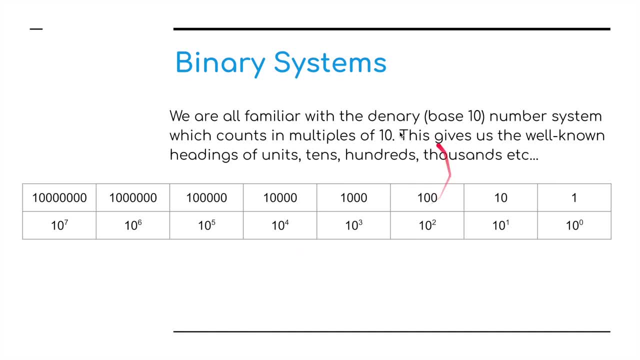 Simply ones and zeros. Obviously, in the base 10 number system we had one, ten, one hundred. Everything's going up. Ten to the zero is obviously one, Ten to the one, ten. Ten to the two: a hundred. 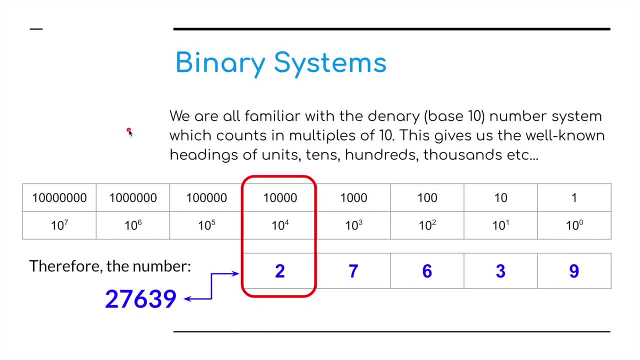 Times in by ten every time. So, for example, in the decimal number system I have the value 27,639,, which would equate to two lots of ten to the four: ten thousand. Seven lots of ten to the three: a thousand. 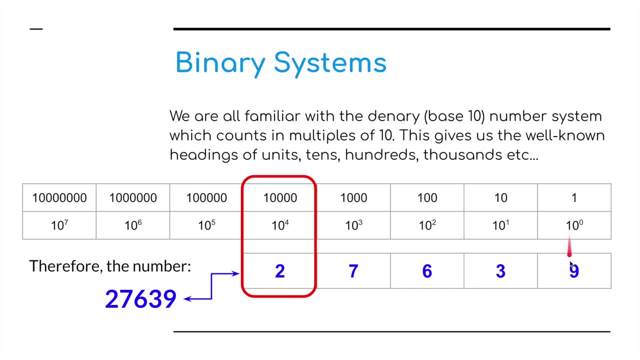 Seven thousands, Six, one hundreds, Three tens And nine units or nine ones. So here we can see we've got two to the four, Which two lots of ten thousand, seven lots of a thousand, six lots of one hundred. 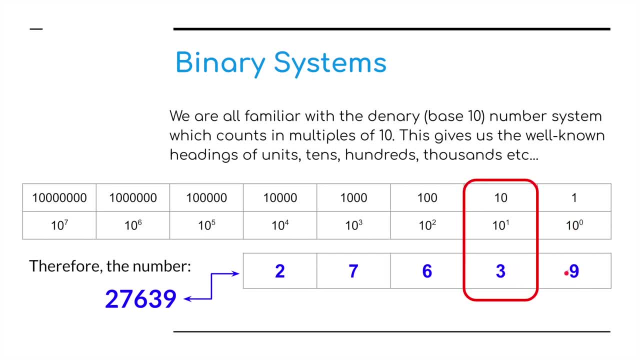 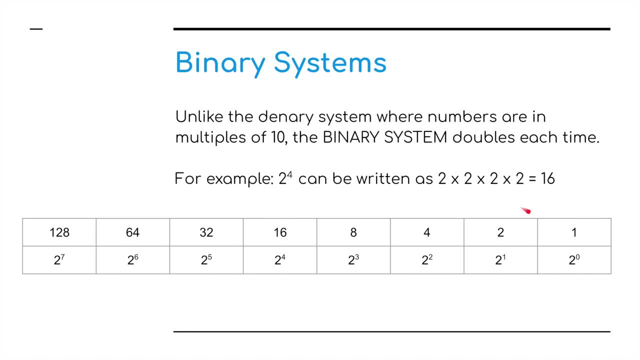 ten lots, three lots of tens and nine units or nine ones. Now. in a binary system these go up in times two, Not times ten times two. So two to the zero is obviously one times two times two times two. 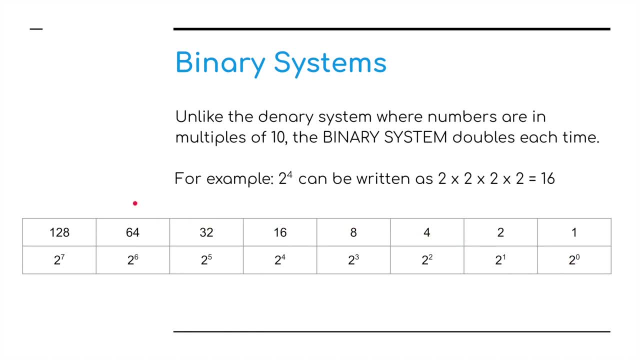 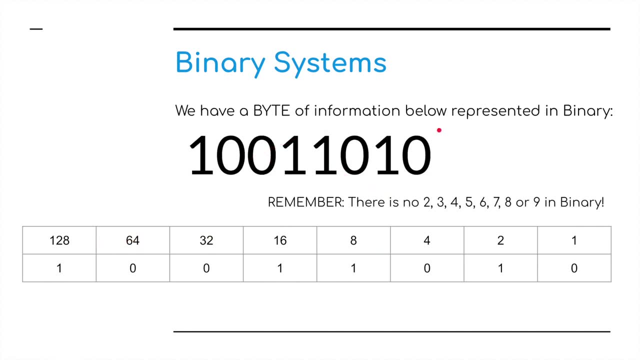 So it's one, two, four, eight, sixteen, thirty-two And, to get to a byte of information, 128.. So let's look at this number here: One zero, zero, one, one zero, one zero. 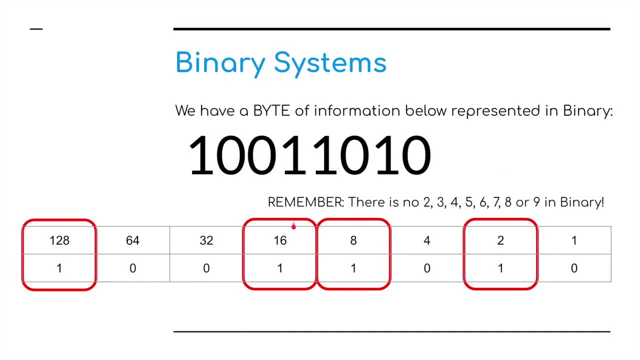 Okay, Well, that's one lot of one to eight, one lot of sixteen, one lot of eight. obviously no lots of four, no lots of sixty-four out of thirty-two and two lots of ones. So if we add all those together we should get a denary value of 154.. 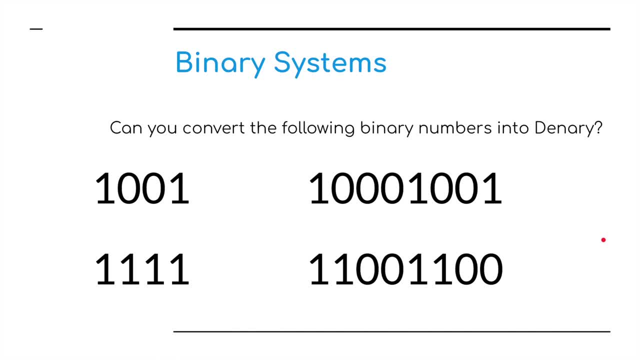 So What I'd like to do? pause the video, have a little go. have a look at the previous slide if you want to have a little go at how you would convert these. I will share the answer with you whenever you're ready. 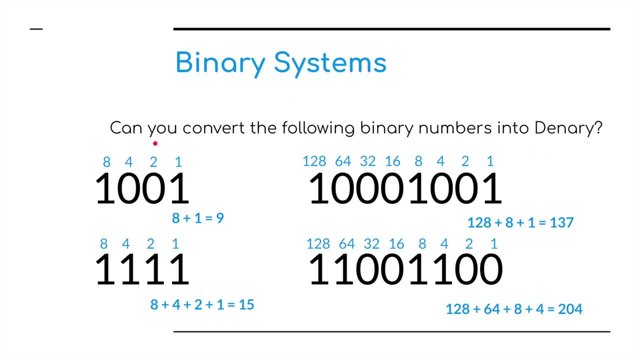 Okay, So obviously the first one, one lot of eight, one lot of one, is nine. This one, one eight, one four, one two, one, one fifteen. The next one, one lot of one to eight, plus one lot of eight, plus one lot of one, is one three seven. 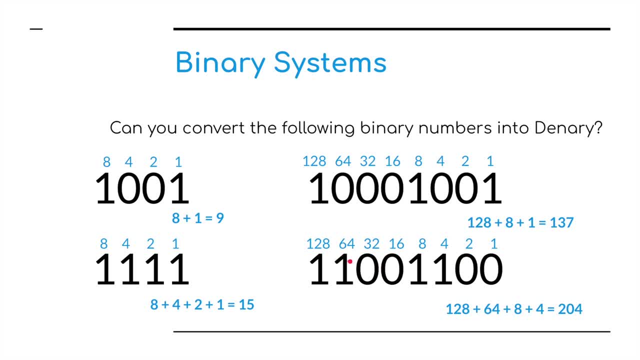 And the final one: one lot of one to eight, one lot of sixty-four, one lot of eight and one lot of four would equal two hundred and four. We're basically adding all the ones together, whichever number they are under. 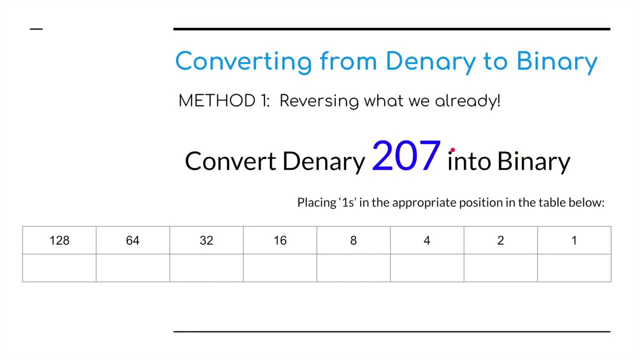 So let's have a little go at this one. Convert the denary value 207, into binary. How do we do that? Well, we put a one under the 128.. Why do we do that? Because we're starting with 127. 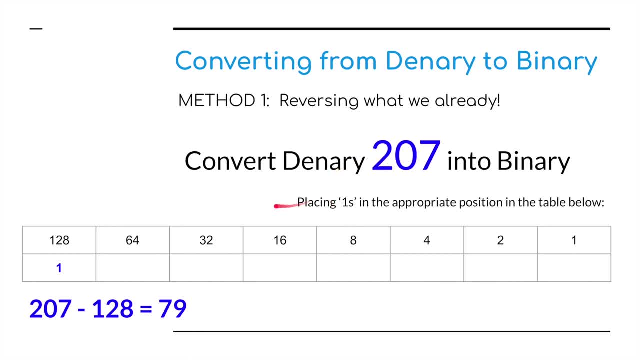 And we're going to put- we're going to see what number's in here- A little bit like in primary school, when you're working with coins and you want to get your change or you want to use your coins to add up to a certain total. 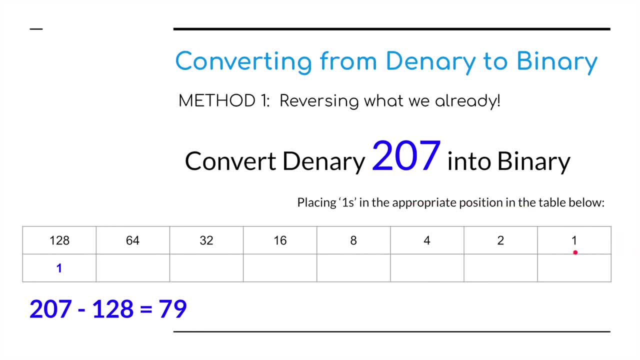 We're going to do the same here. If we pretend we've got a coin with a value of one, a coin with a value of two and so on and so forth, up to one coin with a value of 128, we can only use one of these one coin at a time. 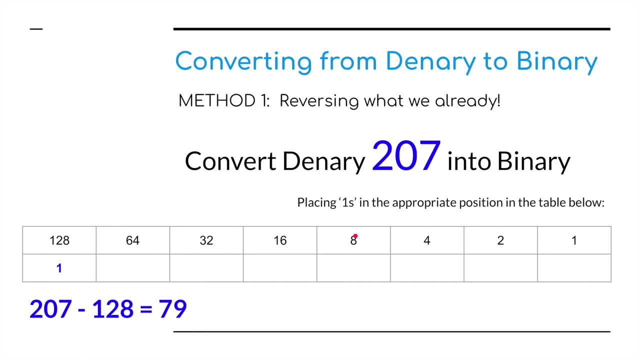 We can't put two lots of 128 in. We're going to use one coin which is 128. So we take that away from 207 to get 79. We'll have one lot of 64, and have 15 left over. 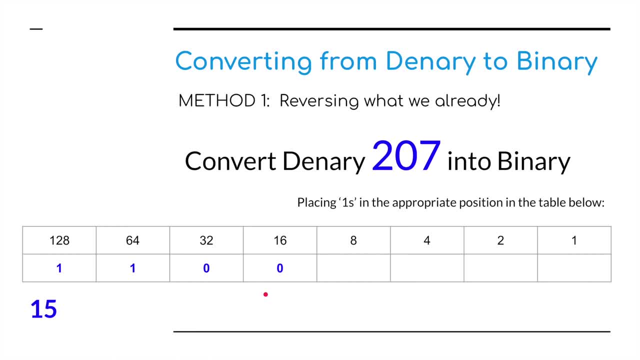 So therefore, we'll have no lots of 32,, no lots of 16,, but 8,, 4,, 2, and 1 add up to 15.. So we've got one lot of each of those. So the denary value for 207 would be 1100.. 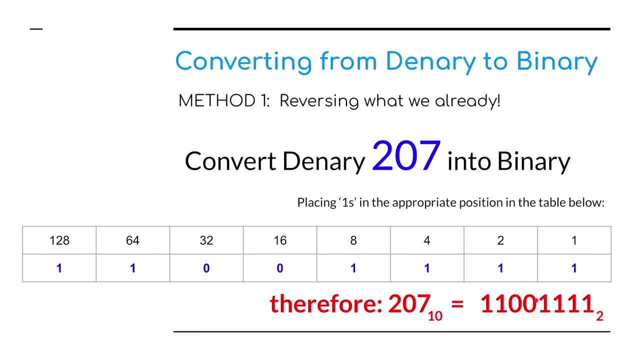 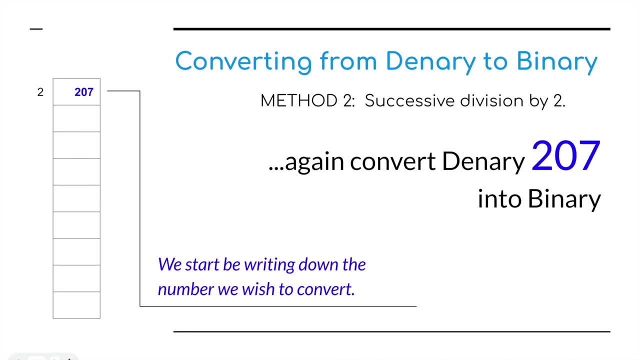 So that's 1111, like. so Okay, there is another method which I'll share with you now. Method two is successive division by two. So we start off with the denary number and we divide it by two. 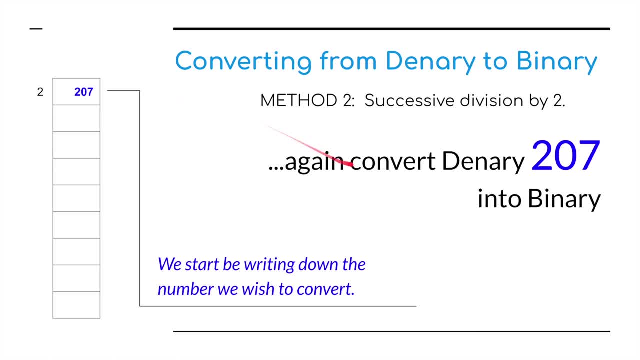 What we're doing here is we're going to be looking for the remainders. So we start by writing the number down. we wish to convert 207.. We divide it by two. We get a remainder one. Okay, so there's two lots. 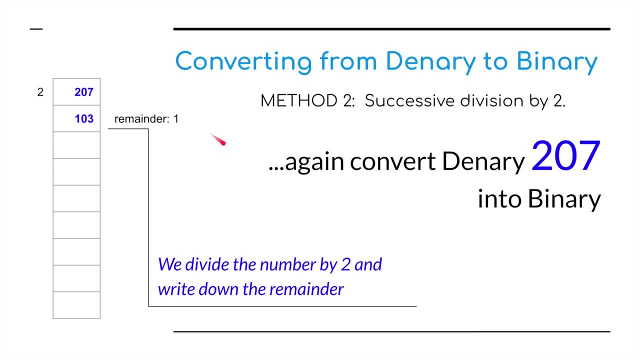 Lots of 103 in 207, with one left over. We carry on dividing it by two. again, We've got a remainder one there, Divided by two. we've got a remainder one Divided by two. again we've got a remainder one. 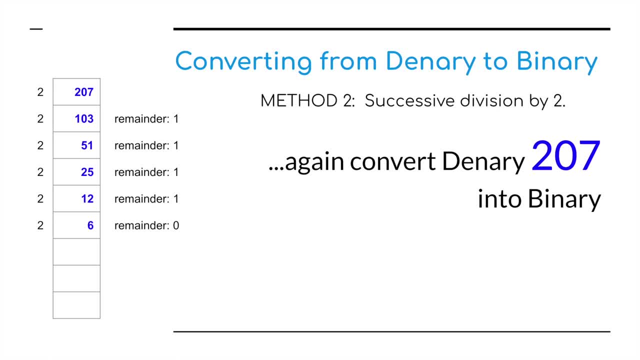 12 is obviously an even number, so we're not going to have any remainders there. Six is an even number, no remainders. Three is an odd number. it's got a remainder And one. obviously we can't divide that by two, so that's got a remainder one in there. 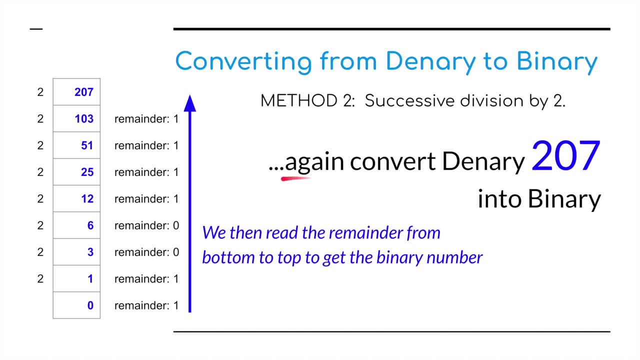 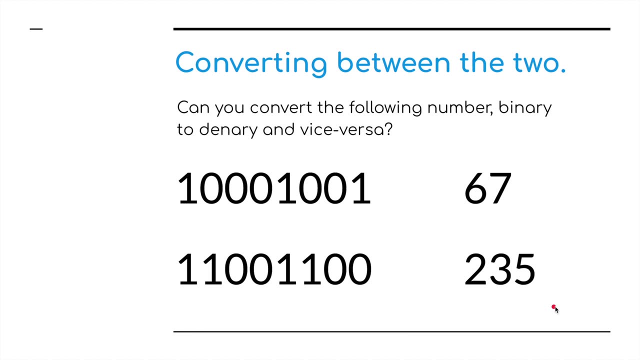 Okay, So we'd read from the bottom and basically the number is 1111001111, which, as we said before, is what we had originally. Okay, so if you want to have a go at these numbers, doing it that way, 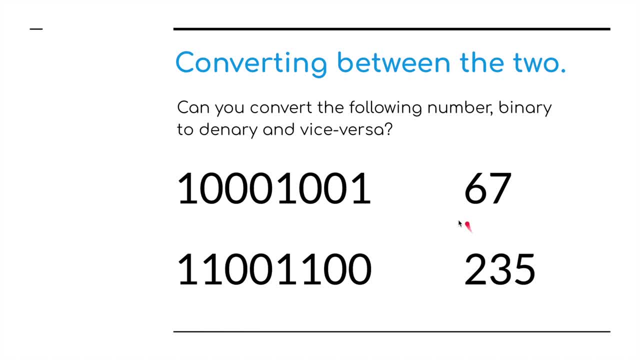 please have a little go. Try both binary to denary conversions and denary to binary conversions there. I'll give the answers As soon as you are ready. please pause the video while you have a little go, And there are the answers. 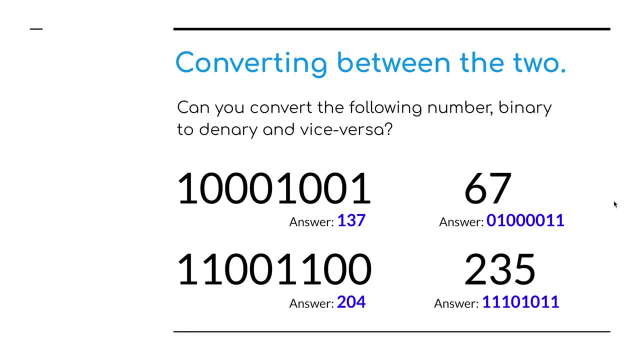 137,, 204, and then we've got 01.. I've written it as a byte of information, ie eight characters, eight numbers: 01000011, or 67, and 235 is 11101011.. 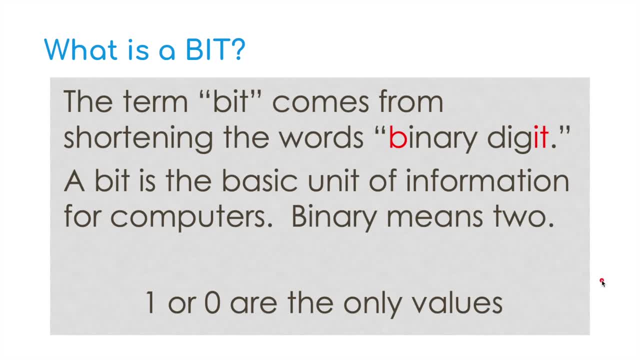 That is it Just to recap One a couple of terms we've used in this video which you may not be familiar with. A bit- the term bit comes from a shortened version of binary digit. A bit is the basic unit of information for computers. 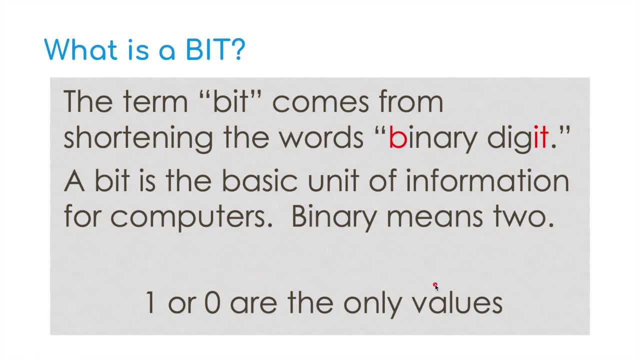 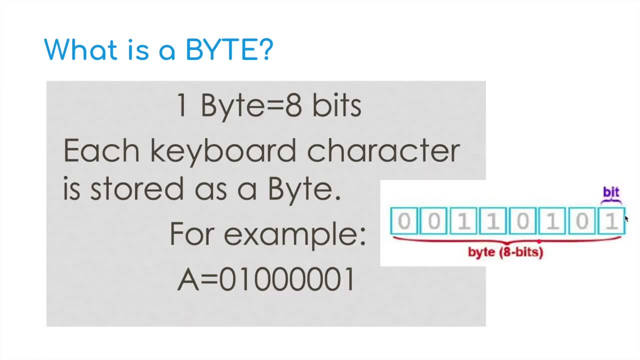 Binary means two, of course, so it's the one or the zero value, two being one or zero. And then a byte I've got to show you. here is- and we mentioned this before- basically eight bits joined together. A string of eight bits equals a byte. 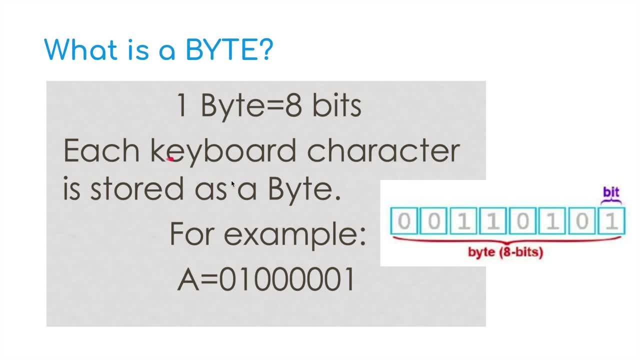 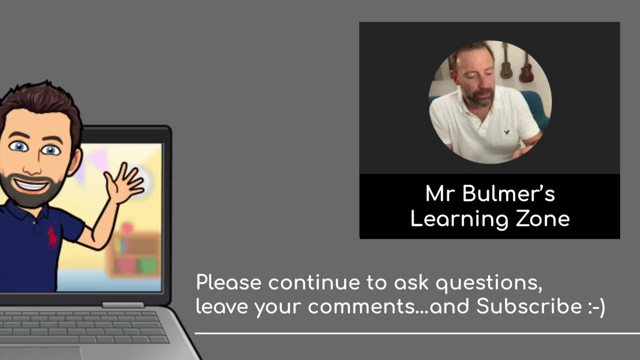 So each keyboard character is stored as a byte Again. we'll get on to ASCII a little bit later on. So, for example, the value A is stored as 01000001,. more about that later. Okay, That is it, ladies and gentlemen, for this first video. a whistle-stop tour of binary. 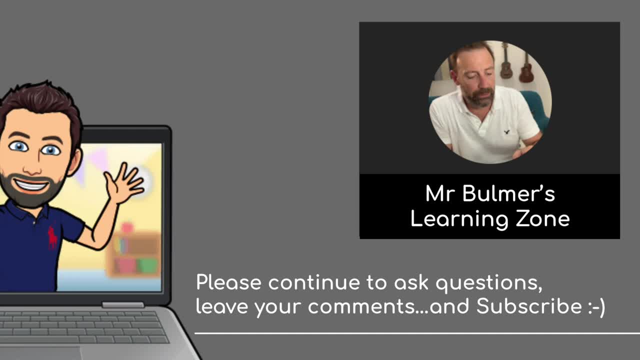